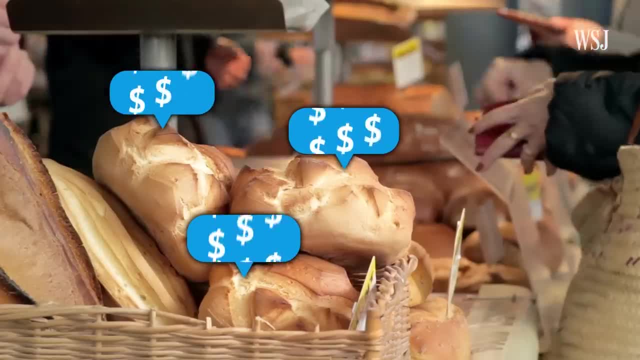 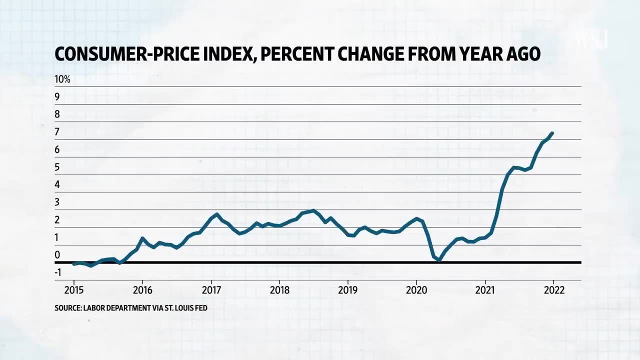 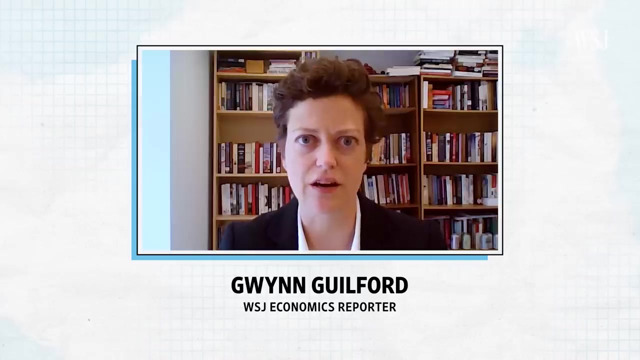 Plane tickets, gasoline, groceries. Inflation has hit the US hard. In 2022, the Consumer Price Index rose at its fastest pace in more than four decades. So the CPI, as it's more commonly known, is pretty much the most closely watched indicator of inflation in the US and consequently, the 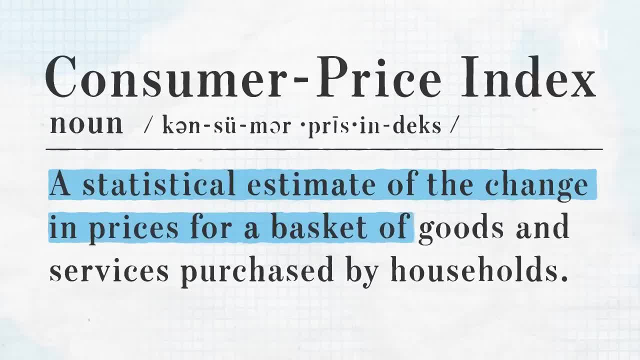 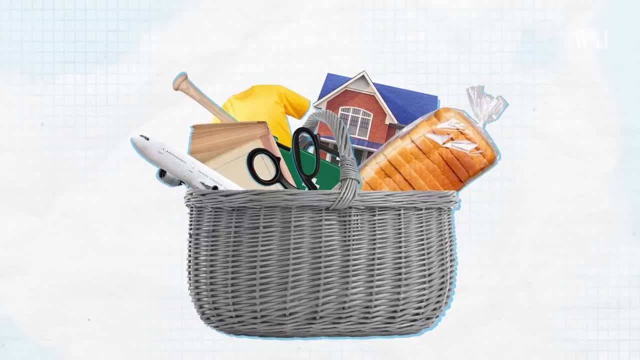 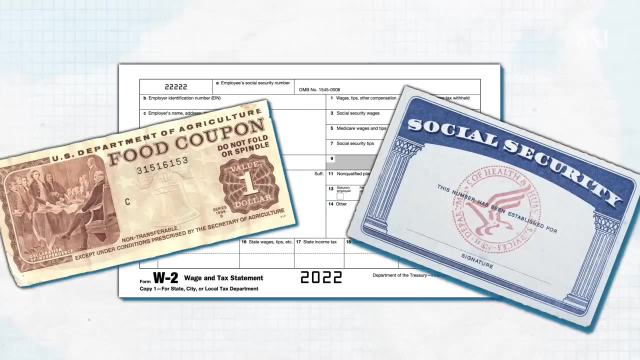 world. The Consumer Price Index estimates the change in prices for a basket of goods and services that represents the average household spending. Calculations made from that basket are used to make decisions that affect Americans all over the country- Decisions about adjusting tax brackets and benefits like Social Security and food stamps- And it's one of the indexes watched. 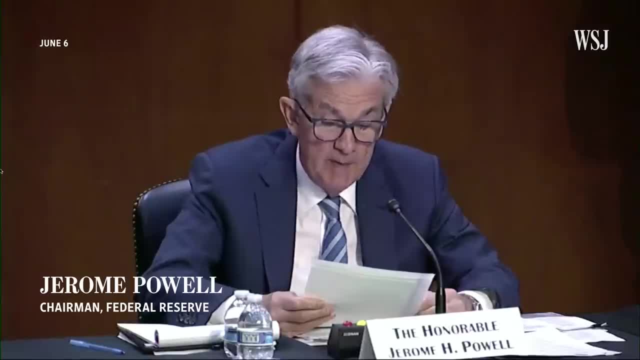 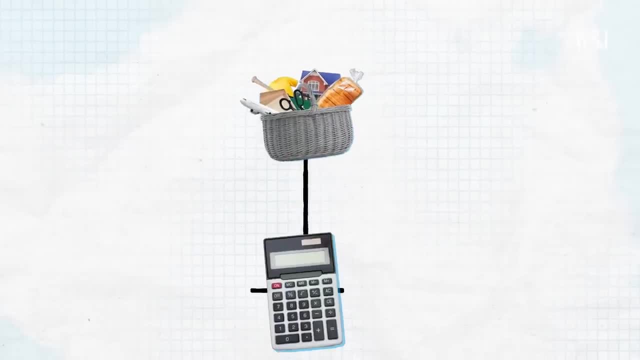 by officials at the Federal Reserve. Against the backdrop of the rapidly evolving economic environment, our policy has been adapting and it will continue to do so. But how is this basket selected and used to calculate the CPI And when shaping policy decisions? why does the Fed pay? 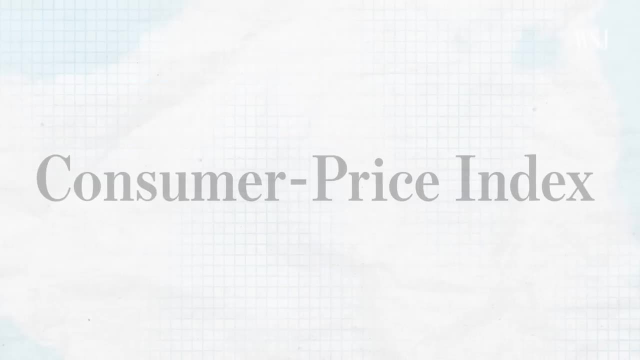 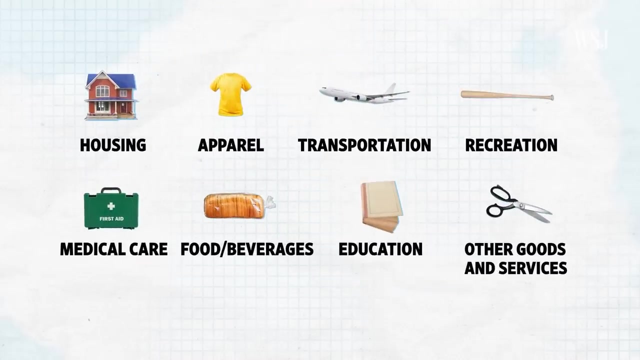 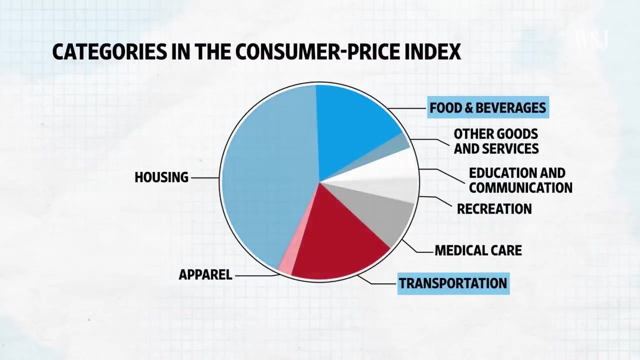 the most attention to a different index. The department in charge of the index, the Bureau of Labor Statistics or BLS, looks at several categories, each given a different importance to compute the month's percent change. Some of the most important categories are food, transportation and housing. 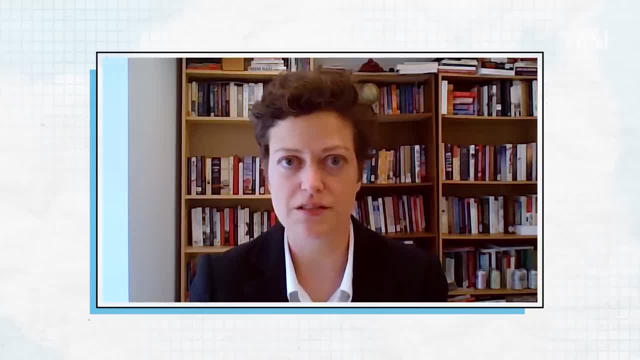 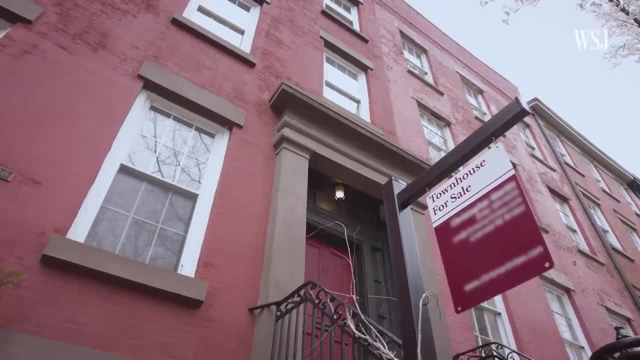 When you pull that all together, housing is a big — I mean, it's the biggest expense that we pay for out of pocket — rent your mortgage. that's going to be, you know, a hefty chunk, more than anything else. 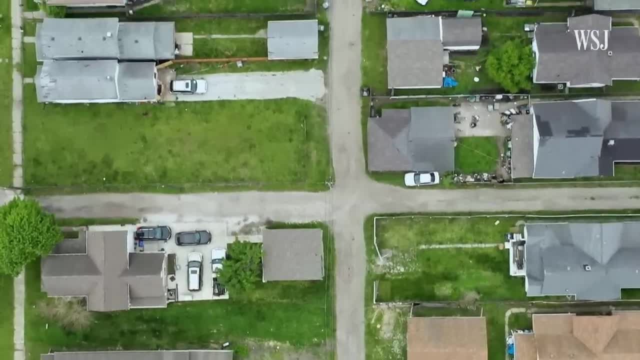 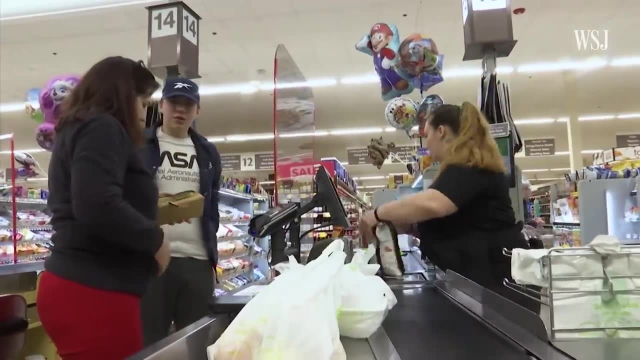 BLS gives each category its relative importance, based on a survey of what consumers buy. Keeping track of all of those items people spend money on, and their price changes month to month, is the job of the BLS's price checkers. The agency employs over 450 workers. 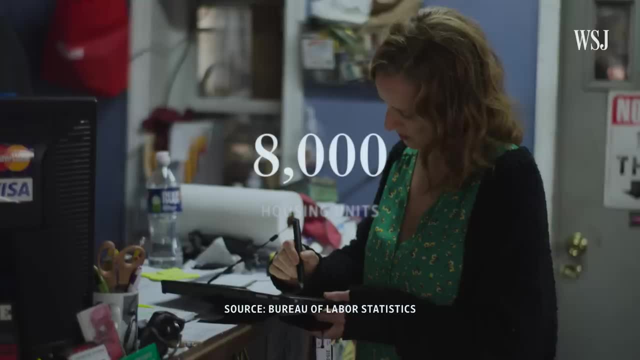 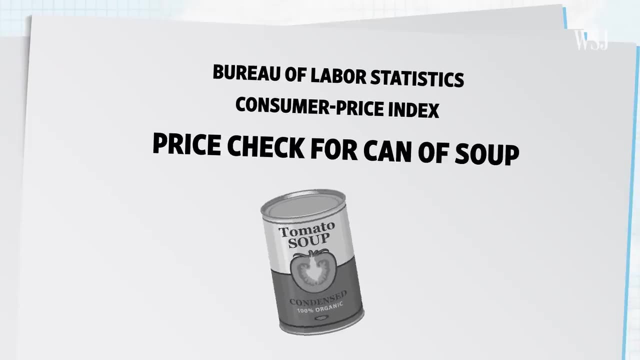 who track prices for up to 100,000 goods and services and 8,000 housing units every month, based on the survey of what consumers are purchasing. To make sure products they are price tracking haven't changed, they compare the product to a list of data points from the month before. 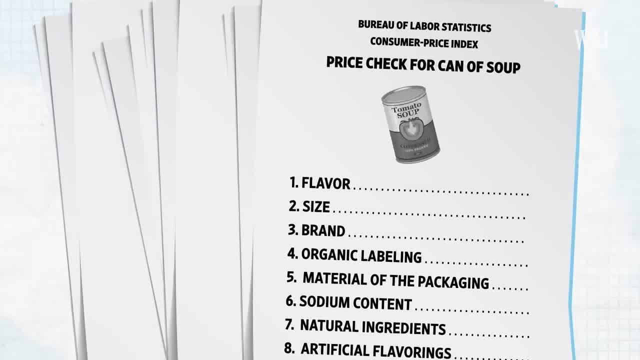 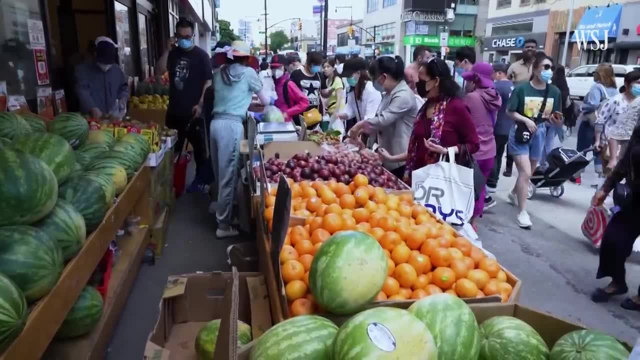 Sometimes that list can be up to 11 pages. This process helps to ensure the CPI's accuracy. The BLS is basing those calculations off of an urban consumer paying out of pocket. The formula excludes non-direct spending, like payments from nonprofit organizations. 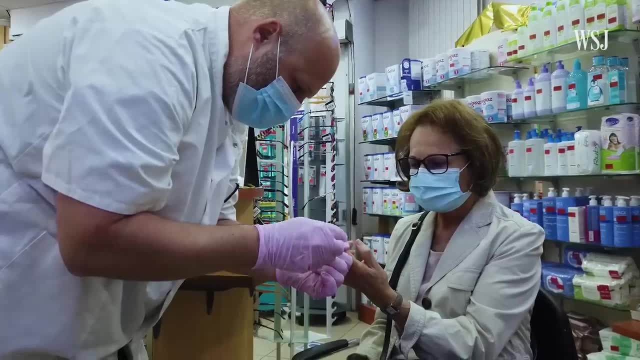 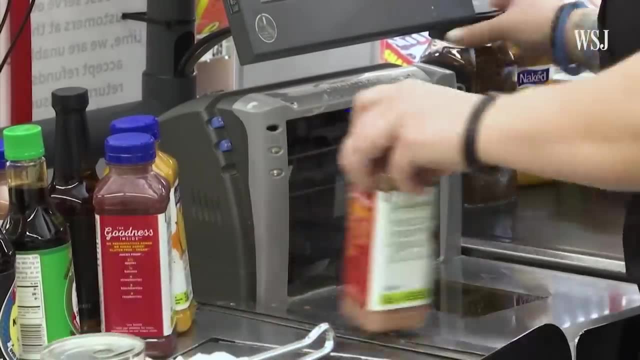 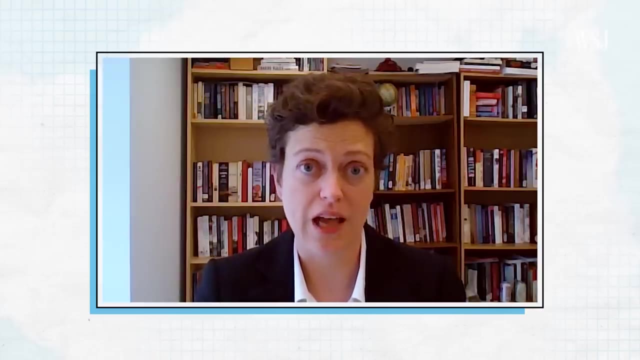 that provide services to households: Medicare and Medicaid and employer-sponsored healthcare plans. But again, this is just an average. Inflation affects different people differently. How you feel inflation depends a lot on what's in your spending basket and how that differs from the average persons. 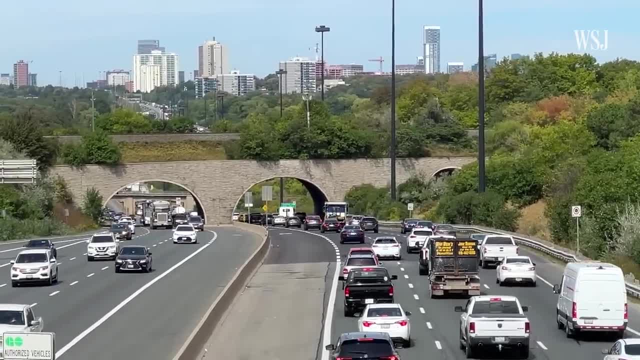 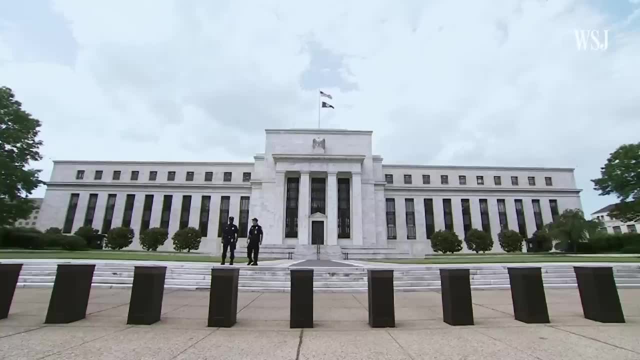 as captured in the CPI. If you have to drive to work every day, you are feeling inflation a lot more than the person who has to take the subway, because gas prices have gone up so much And the index doesn't include everything. That's why some like the Federal Reserve. 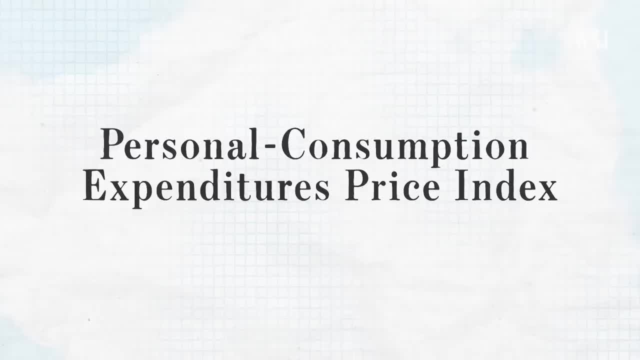 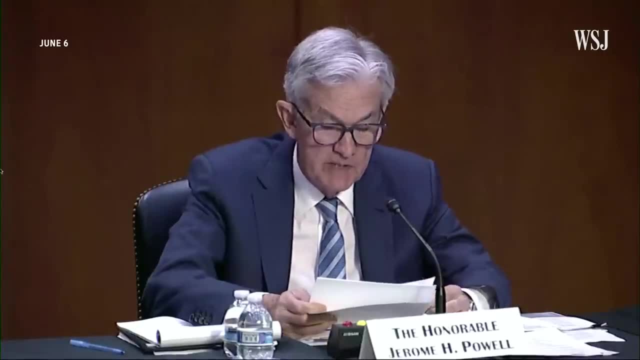 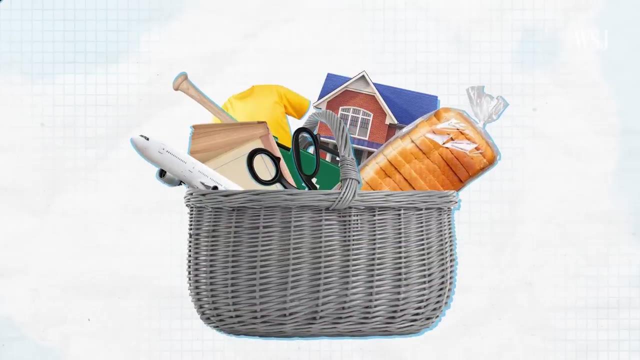 prefer indexes they see as broader, like the Personal Consumption Expenditures Price Index, or PCE. Over the 12 months ended in April, total PCE prices- that's, Personal Consumption Expenditures prices- rose 6.3%, One of the reasons the Fed prefers this index. 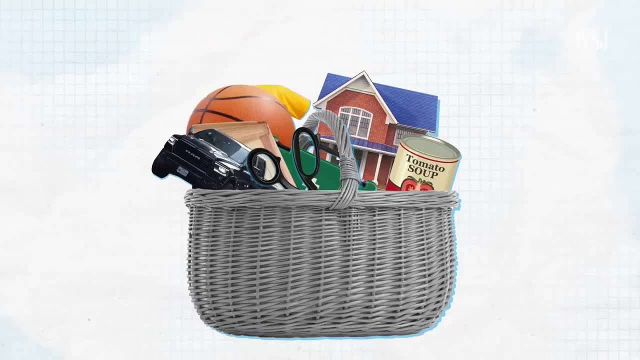 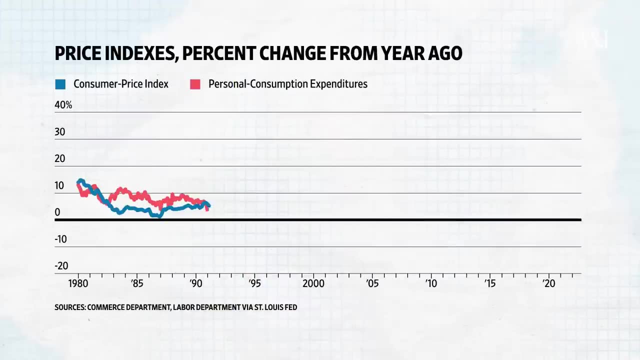 is that the CPI only transitions items in and out of the basket every two years, while the PCE changes its basket month to month based on consumer trends. The variations in how CPI and PCE are calculated mean that the two indexes can reflect American inflation. 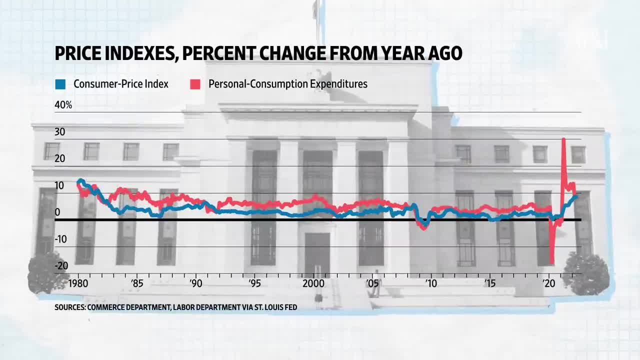 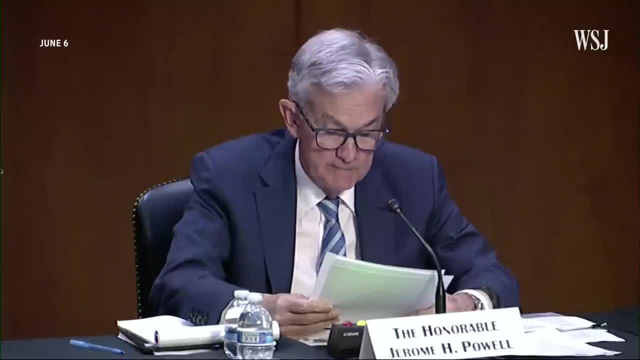 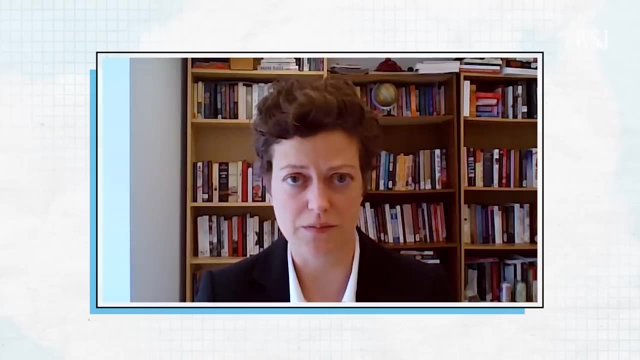 slightly differently, but the Fed takes both into account. The Fed's monetary policy actions are guided by our mandate to promote maximum employment and stable prices for the American people. Looking at multiple indexes gives the Fed a broad picture of American inflation. CPI is undoubtedly something. 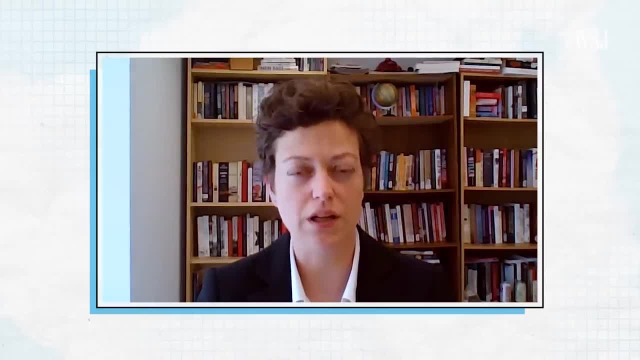 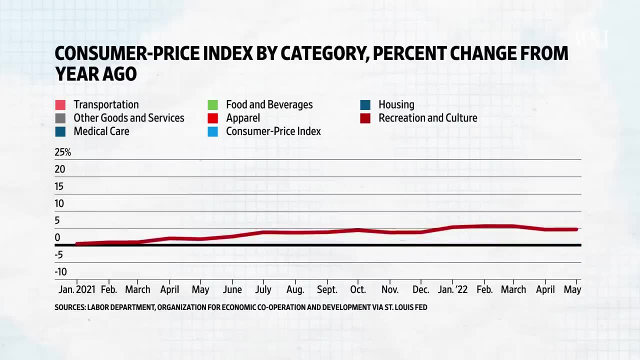 that they're watching closely, especially the month-on-month movement, Like that's an important gauge of you know it. does this inflation we're seeing does it have momentum? And rising inflation of vital items, especially over long periods of time, can cause more issues. 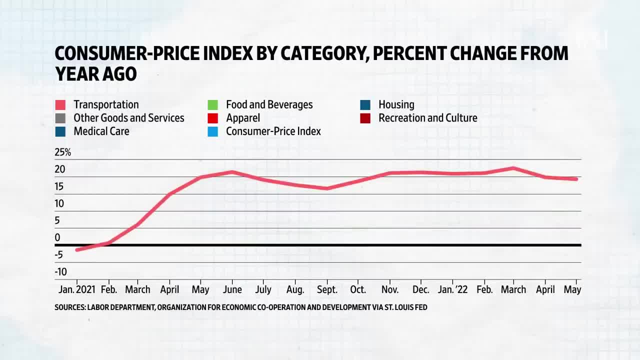 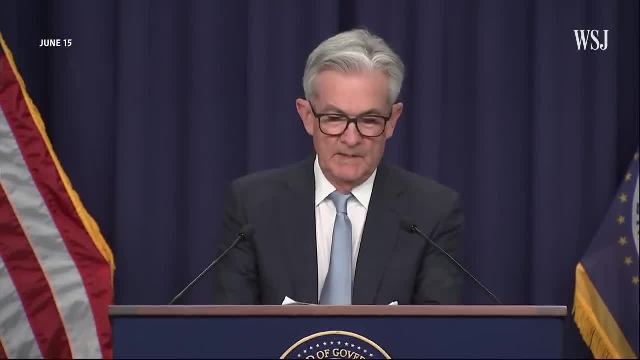 like inflation becoming embedded in the economy. We at the Fed understand the hardship that high inflation is causing. We're strongly committed to bringing inflation back down and we're moving expeditiously to do so. When inflation remains high for too long, consumers begin to change their behavior. 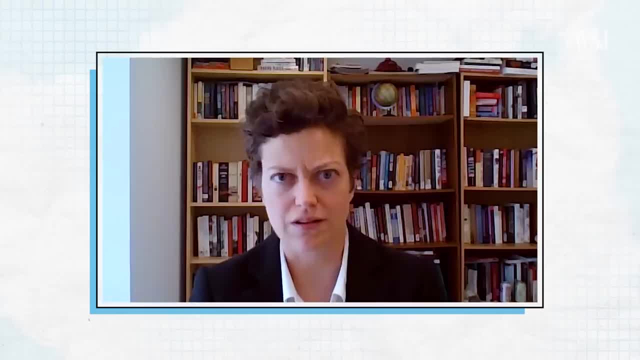 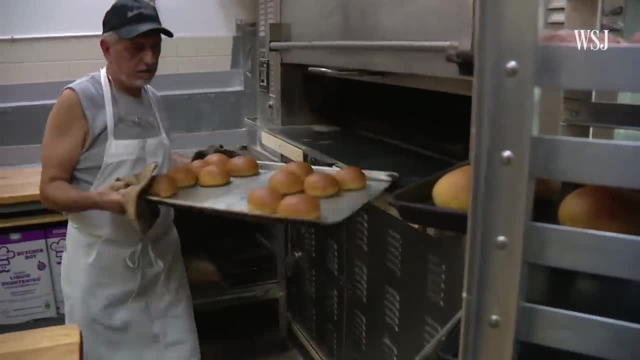 in ways that can keep prices elevated. So, for instance, like: ugh, my bills are getting really expensive, so I'm gonna ask for a raise. And then your boss is like: people seem to be willing to pay my higher prices. 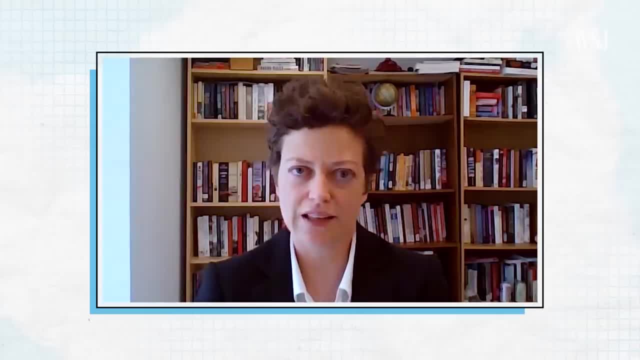 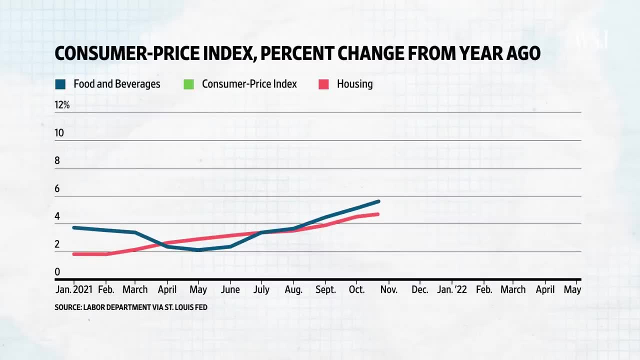 so I'll just give this person a raise And raise my prices. That keeps inflation kind of chugging along in a way that you know can be eventually harmful for the economy, By looking at changes to individual categories like housing and food. 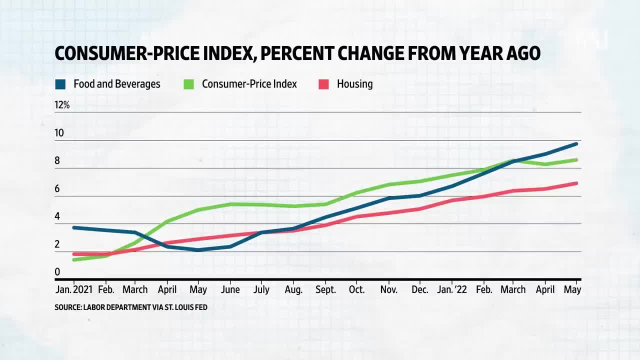 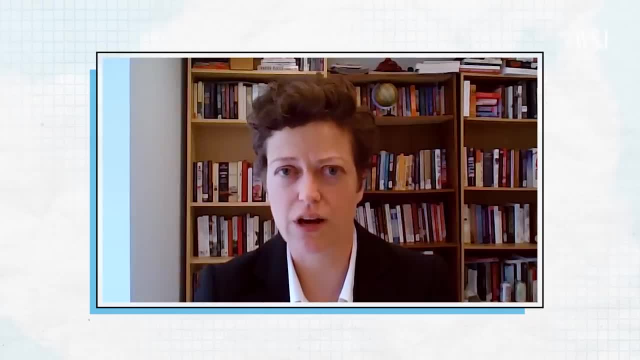 consumers can learn specific information from the overall CPI. That's gonna give you a sense of whether inflation is broadening, and that's really the concern right now for the economy. The CPI is a useful tool for economists and consumers alike and it's a good indicator of whether inflation will. 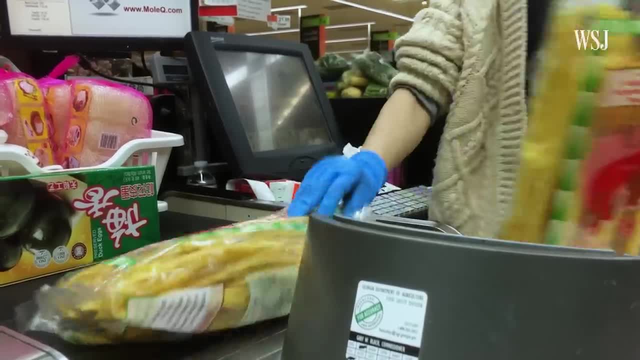 begin to subside, or whether it will become more embedded in the economy. 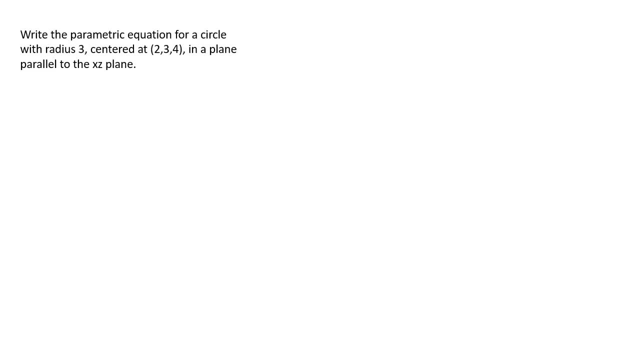 So we want to write the parametric equation for a circle with radius 3 centered at the point in a plane parallel to the x-z plane. So let's start visualizing this in 3D. So here's my x, y and z axes and our center. 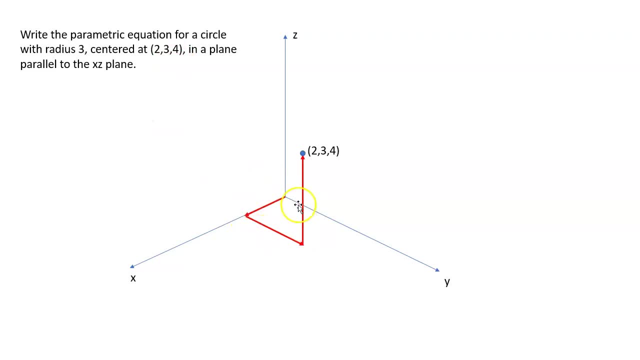 point would be at 2 in the x, 3 in the y, 4 in the z, and I'd have my point in 3D space there. Now our circle lies in a plane parallel to the x-z plane. Now the x-z plane is the plane that contains the x-axis and the z-axis. 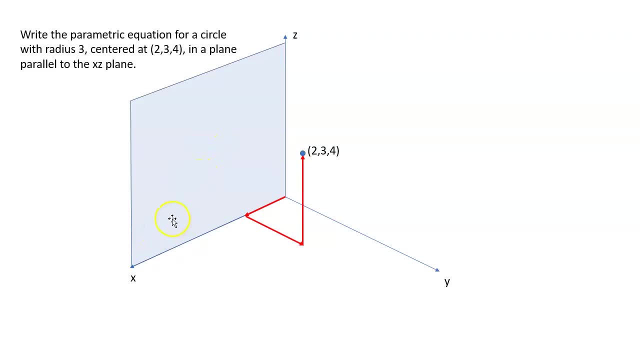 where y is equal to zero. But we're talking about a plane parallel to this and presumably we're going to want it to include the center of the circle, So we're going to have to shift that plane out to a y value of 3.. 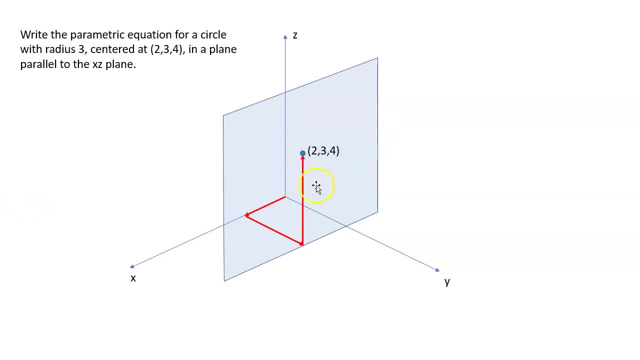 So this plane would be the plane. y equals 3 if we needed to write that for some reason. But the important thing to note is that x and y can be changing, but sorry, x and z can be changing, but notice that at any point in this plane y is. 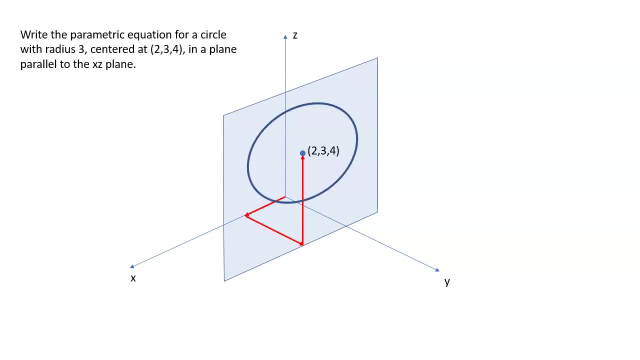 going to be constant at 3.. So now let's introduce our circle. So now we have a circle with radius 3 centered at that point and you'll notice that the is happening in x and z. Again, remember, y is constant here.